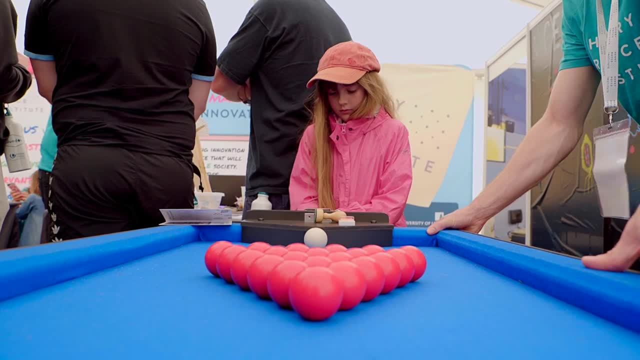 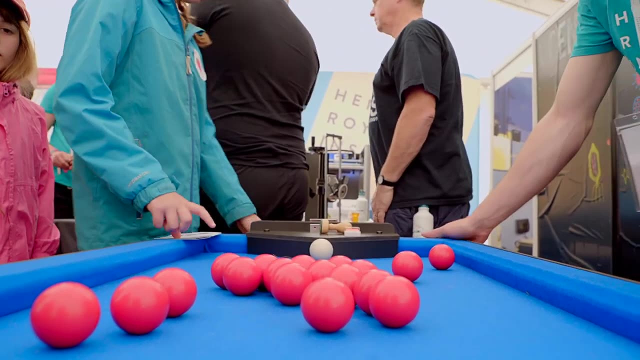 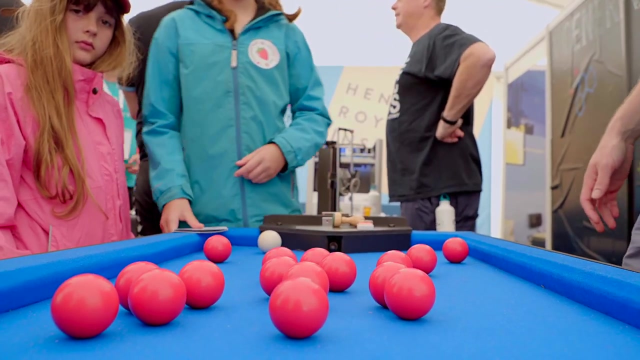 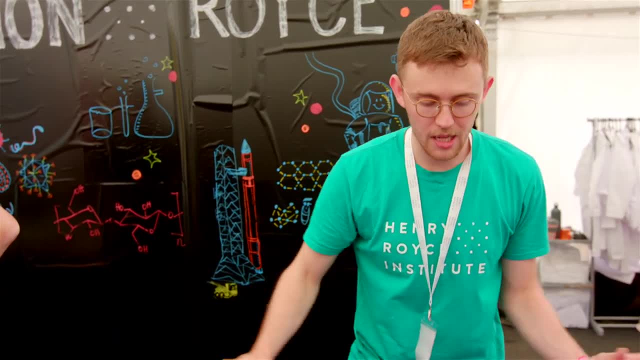 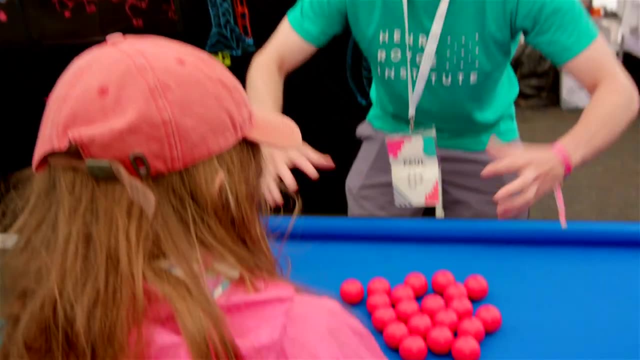 to what they were like before. They've all scattered. Yeah, exactly, They've all spread out. So the atoms, they've all spread out. They want to try and get back to each other. They want to try and get into that tightly packed arrangement. 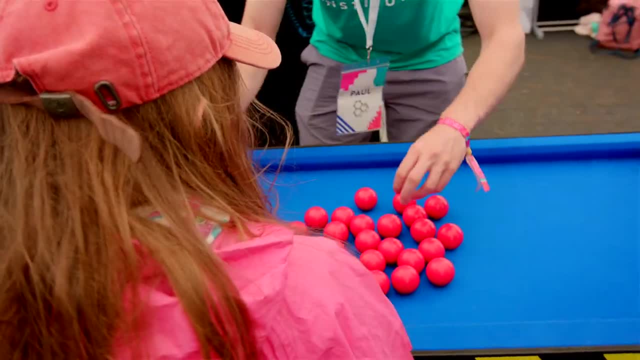 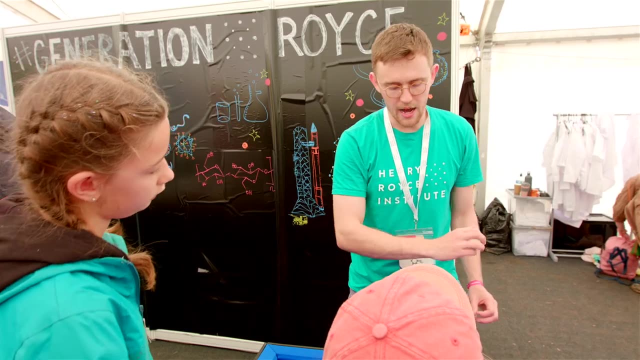 they were in before, But they can't quite do it. They leave gaps and bits missing from the structure. And as more and more neutrons keep firing through and firing through inside this nuclear reactor, the gaps get bigger and bigger and bigger. And you've got these. 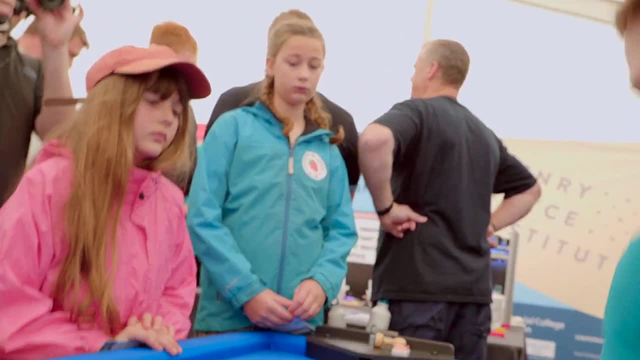 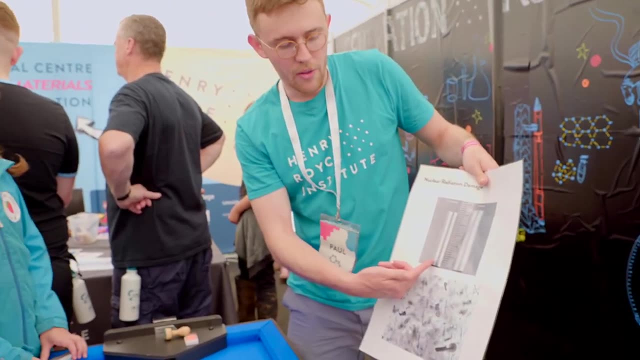 empty spaces for them. So what do you notice about what's happened to the atoms and what's forming? So, even though the atoms themselves are too small, the effects can be seen in objects in real life. So can you tell me the difference between the bar on the left and the bar on? 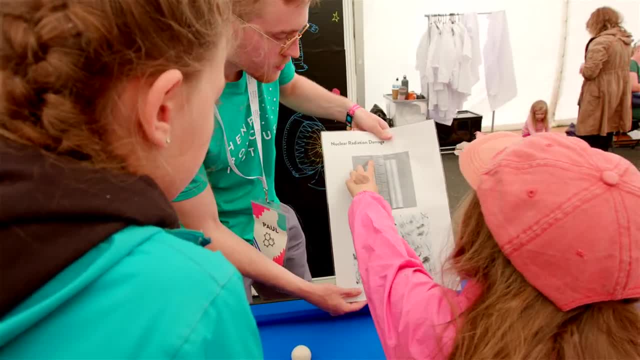 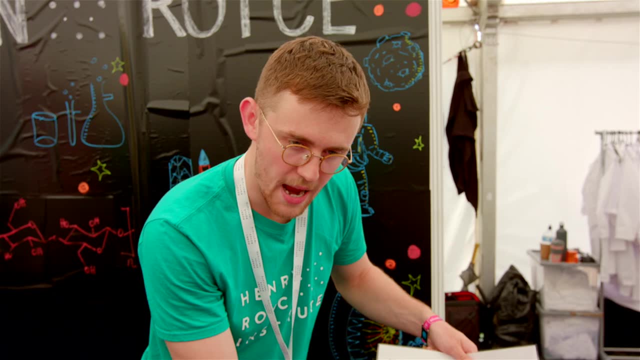 the right, That one's thinner and it's smaller, That one's wider and it's taller, Exactly right. So what if I told you these two bars were actually identical? at one point They were exactly the same size, But then the one on the right went inside one of these. 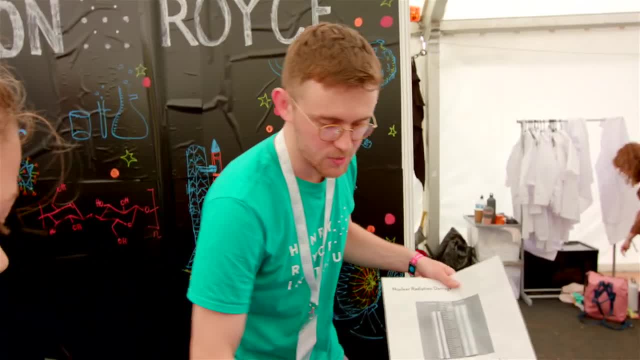 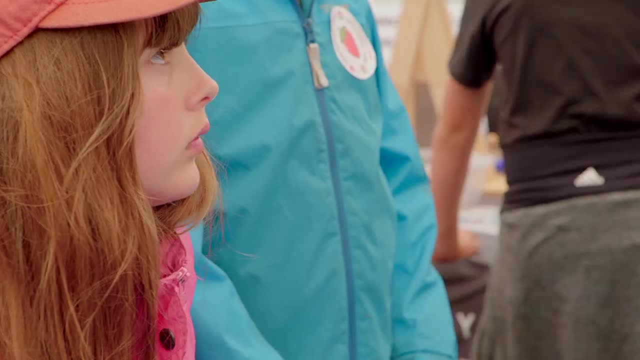 nuclear reactors, The neutrons came out. So what do you notice about that? The neutrons came passing through, smashing all the atoms up and made these gaps inside of it And, as a result, the whole thing's gotten bigger. Isn't that cool? 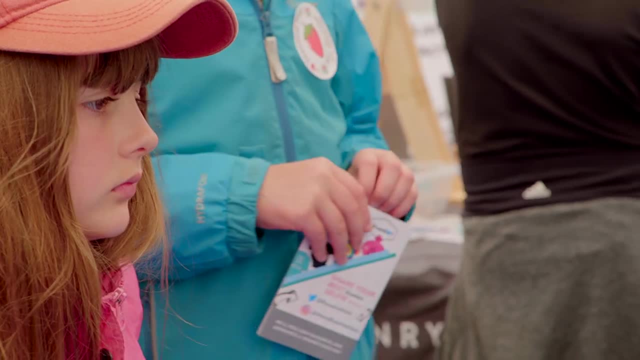 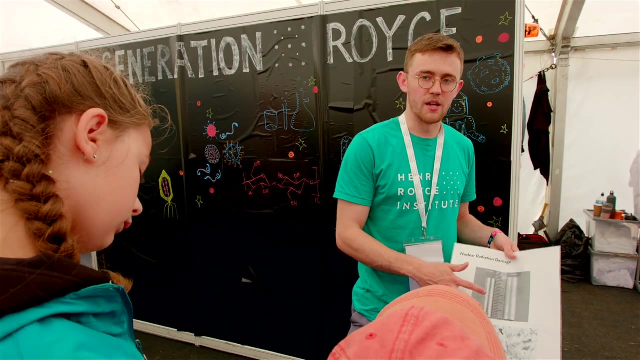 Yeah. So when you're designing nuclear reactors, you have to make sure you understand what happens to these metals, And if they're going to swell up, you don't want gaps forming and things leaking out. So that's why it's very important to understand nuclear material science. So I hope that all made sense to you girls, Yeah.